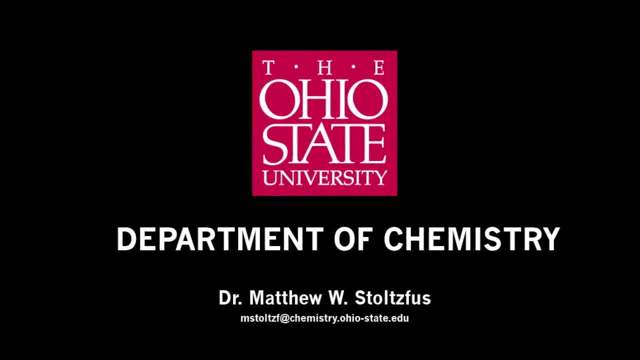 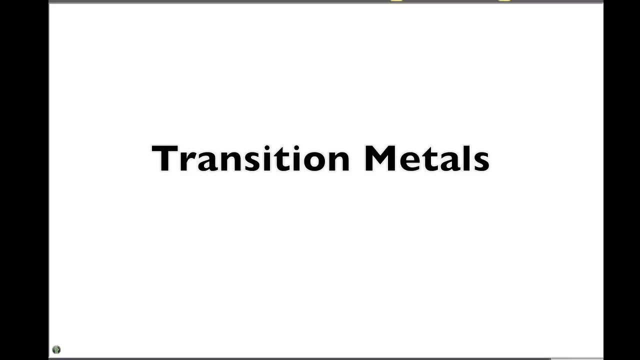 For the compounds that we're looking at, we have- and I'm gonna try to emphasize this and say- an atom versus a molecule. If we looked at nickel as an atom, it's gonna be completely different than Ni, NH3,, 6,, 2 plus. 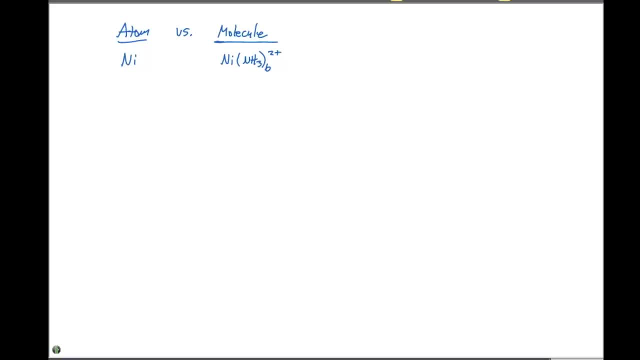 So the system that we use to get an electron configuration for an atom is gonna be different, or in this case, slightly different than what we look at for a molecule. Because, for nickel, if we looked at its electron configuration, if we look at the periodic table, 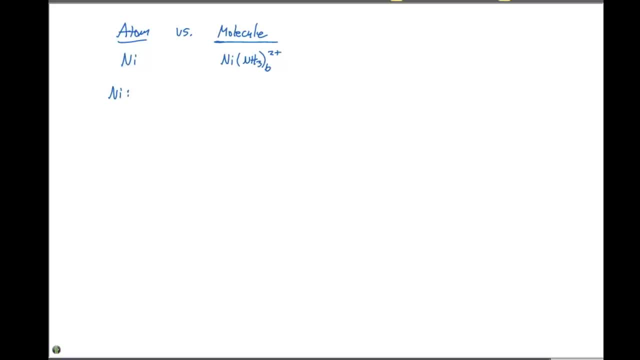 nickel is element number. That means as an atom we need to put 28 electrons into all the orbitals And we're gonna fill that in in the lowest energy configuration possible. So nickel is gonna have the argon core and 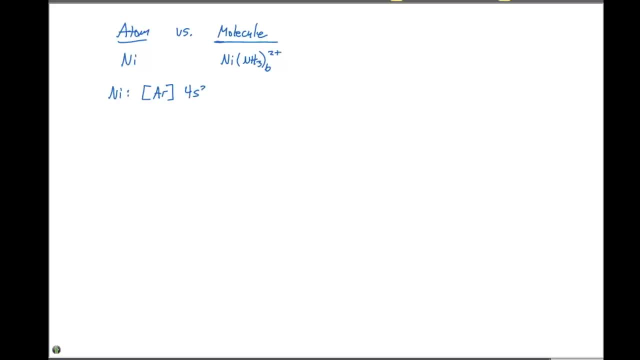 it's gonna have an electron configuration of 4s2, 3d8.. So the next compound that we look at- we're gonna have an electron configuration of 4s2, 3d8. Is nickel: NH3, 6, 2 plus. 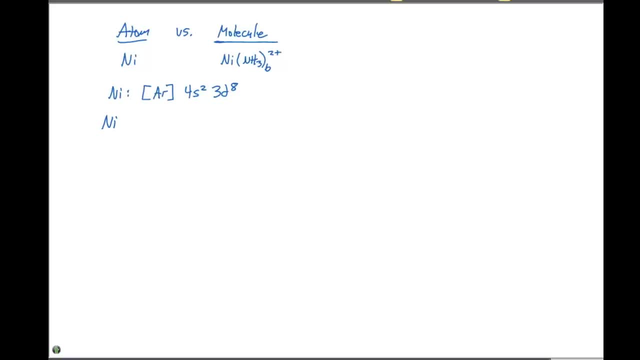 The ammonia ligand is neutral. So that means the oxidation state of the nickel, where the charge of that nickel cation has to be two plus. So the question is, what changes when we go from a nickel atom to a nickel 2 plus cation? 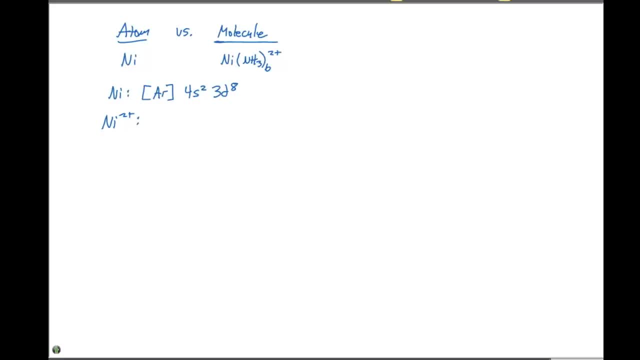 Okay, the obvious answer here is nickel, 2 plus 2 plus. here is we're gonna lose two electrons. okay, Now the not so obvious answer would be which two electrons have to be lost. So if I'm nickel and I have all these electrons buzzing around me, right? 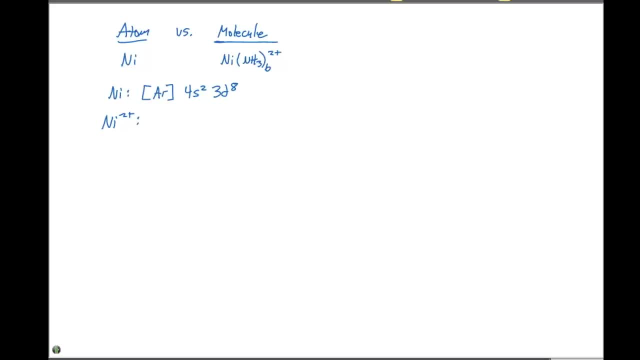 Which electrons are gonna be removed first? Okay, someone said the d orbitals. Anybody wanna take another guess? The s orbitals. okay, So let's think about this. Everything has to do with energy when we're looking at these transition metal. 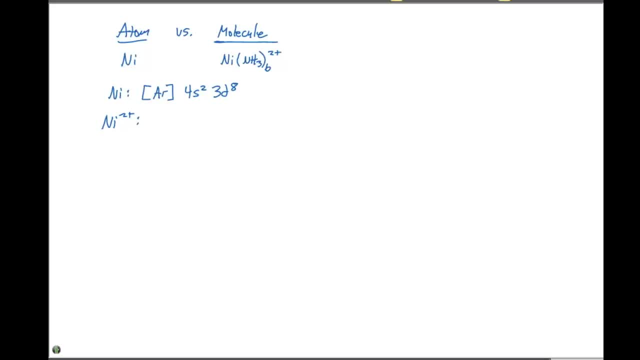 complexes or any type of molecule or ion or atom that has electrons in. So the easy answer is: the electrons that are lost are gonna be the ones that are the easiest To remove. makes sense, right? So it's kinda like if I'm reaching in to grab an electron. 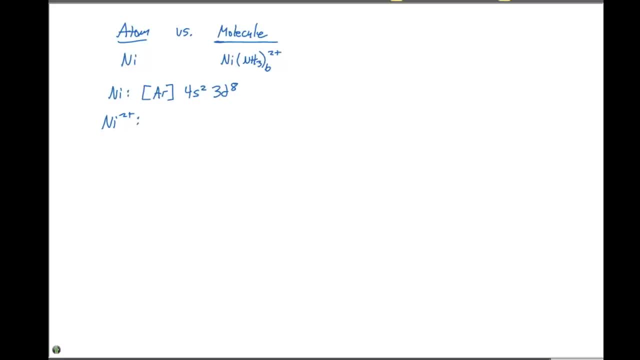 I'm gonna grab the one that takes the less energy possible, okay, Another way of looking at it, that's looking at it from me going in and grabbing an electron and pulling it away. Another way to look at it is if I'm the nucleus down here. 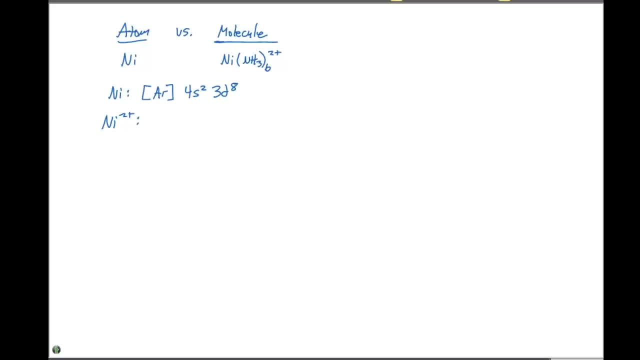 I have my. all my protons were positively charged. okay, The electrons that I'm gonna let leave are: when those two electrons leave, what is the lowest energy configuration that I'm gonna be left with? okay, And it doesn't owe. you should never assume that the way we put the order. 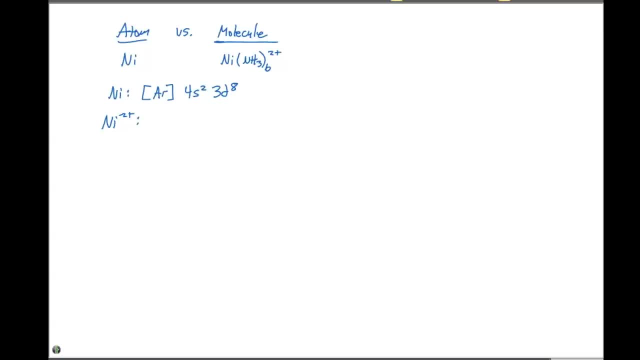 of the electrons in are the way that those electrons are gonna leave in the opposite order. okay, Because what happens here is that the 4s orbital is a really, really large sphere like a basketball. The d orbitals- we're gonna look at the different shapes of those and it just so. 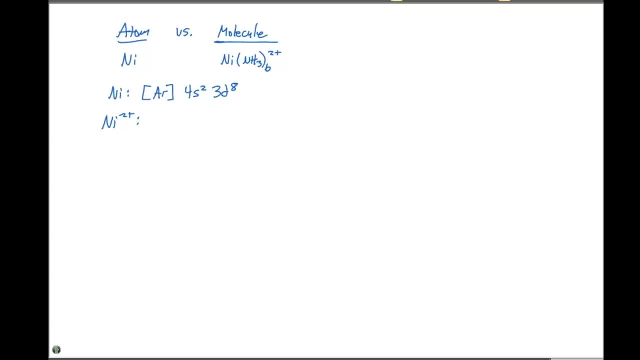 happens that the 4s orbital. The 4s orbital extends farther into space than the 3d orbitals do. If I'm a nucleus and I'm positively charged down here and there's electrons buzzing around out here, If I'm really close to the nucleus, 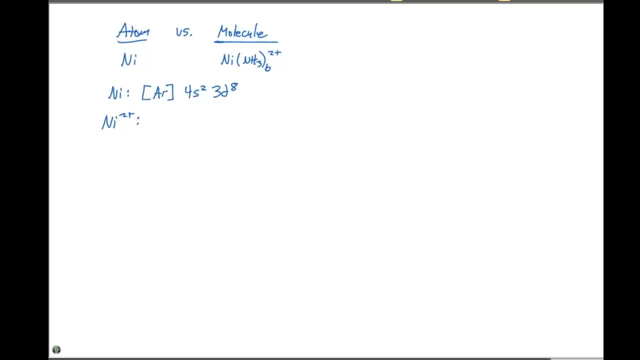 there's gonna be a strong attractive force there. But the farther I go away from the nucleus, the easier it is to remove me. And when you have an atom versus an ion- we also have- we have to take into account what happens with those ammonia ligands. 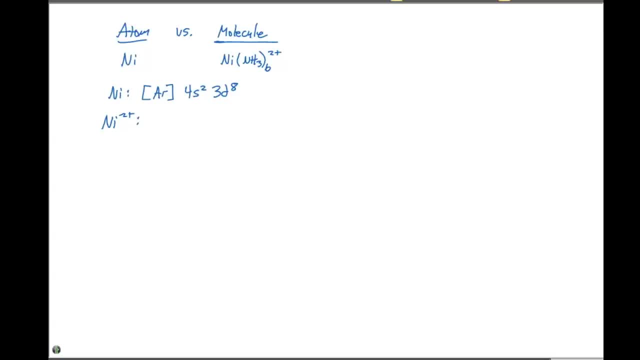 So we're gonna talk about this and the reason for why this is in, probably sometime later this week or early next week. But when I write an electron configuration for a metal cation, I have to say that this is gonna be argon 3d8.. 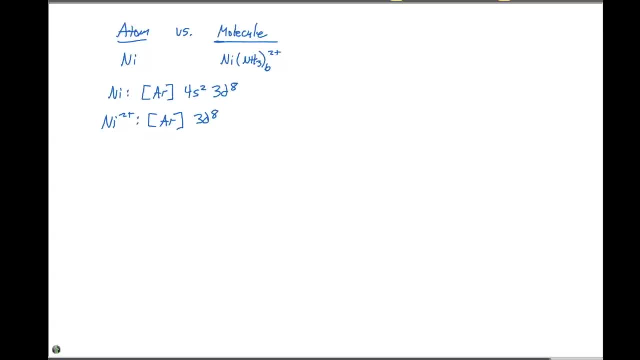 Okay. So The general statement that we can make here is: it is easier, Or we can say it takes less energy, to remove the 4s electrons from a transition metal. So therefore, when we write out an electron configuration, we're always gonna remove those s electrons first. 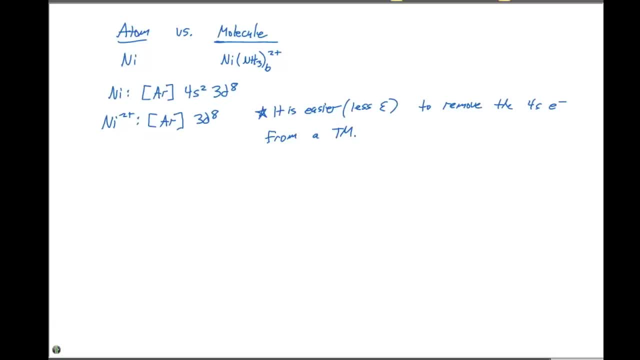 This is the reason that practically every transition metal along the transition metal series has a two plus oxidation state, Because for it to become a two plus charge it has to lose two electrons. So transition metals occur in varying oxidation. The main reason that all of them, or most of them, have a two plus charge. 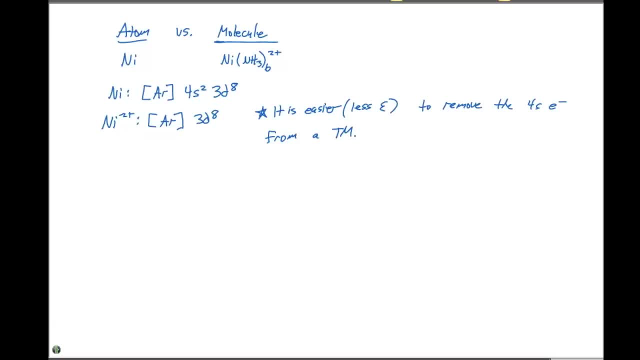 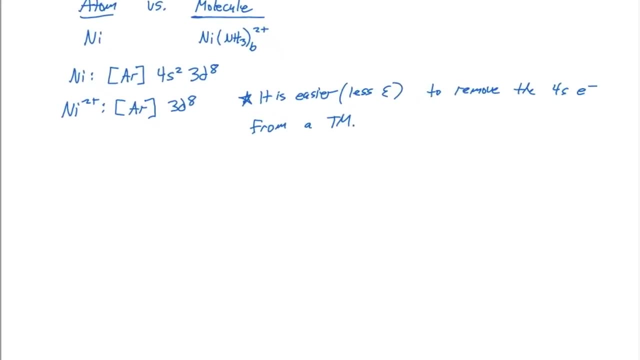 is because it's like, hey, get those electrons in that s orbital out of here. So they're gone, and then we have to analyze a little bit more to figure out if it's a plus three and a plus five, or a plus four or a plus six. 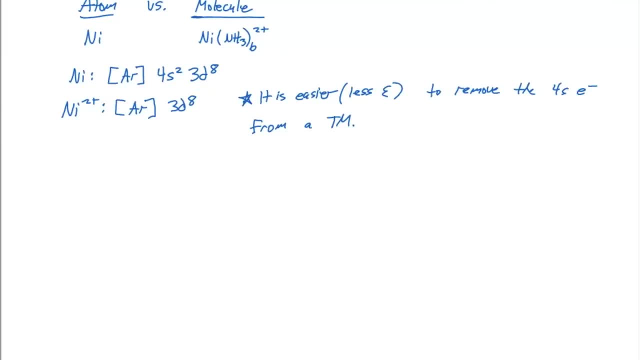 or anything like that. So this is the thing that we have to analyze and this is the general rule: that when we're looking at these kinds of things, these complexes, it's easier to remove the s electrons. So when we're looking at the d electron count, which is very 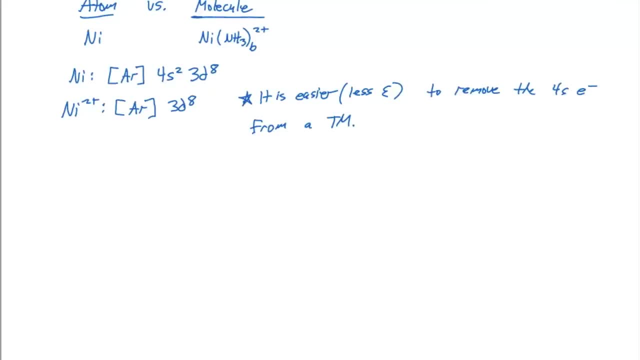 very important for color and magnetism. we need to recognize that. okay, So we can do the same thing then for the cobalt two plus and the zinc two plus. All right, I'm gonna go through and do zinc. If we looked at zinc as an atom, it's gonna be argon 4s2, 3d10. 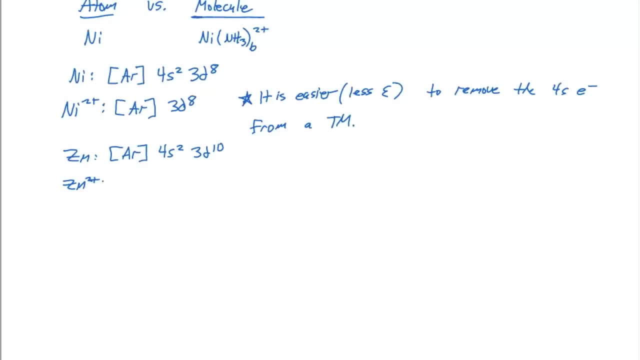 When we have zinc two plus we have argon 3d10.. And what I want you to try to recognize and try to link here- and we're gonna talk about this later- Is that what is special about a d10 case.